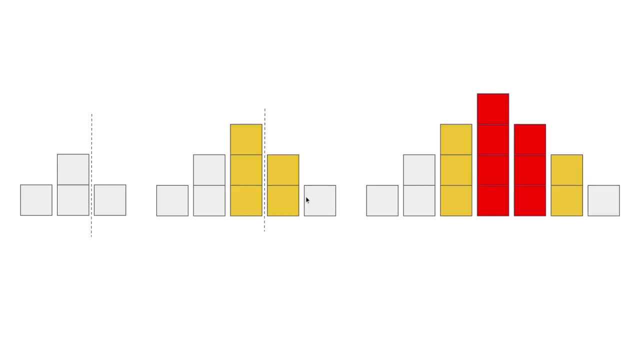 This is the first fifth perspective. I split it at this position And we put one more layer higher stack And to keep this, to keep the original, to keep the symmetry, And we add another seam-hide stack, So… for the third one, we do the same. 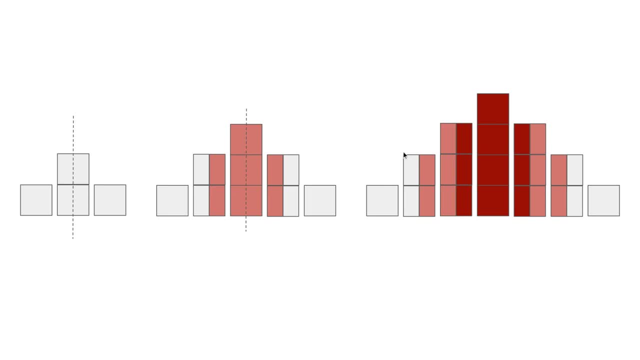 Sixth perspective: we call it porting of the Red Sea. It's actually a geological concept. It's like a rifting in the middle and new volcanic rocks form like new land or fill the space in the middle. so you can see it's like 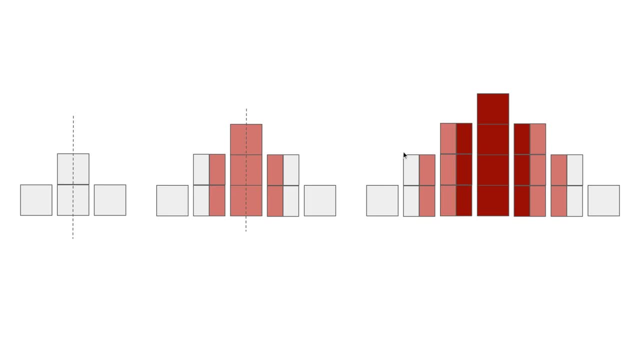 a rifting and new land formed. So this is the seventh one. The seventh one is my favorite perspective. It's like a volcano and the middle column of squares grows high and the rest follow like lava in interacting from a volcano. This is this one is my favorite one. 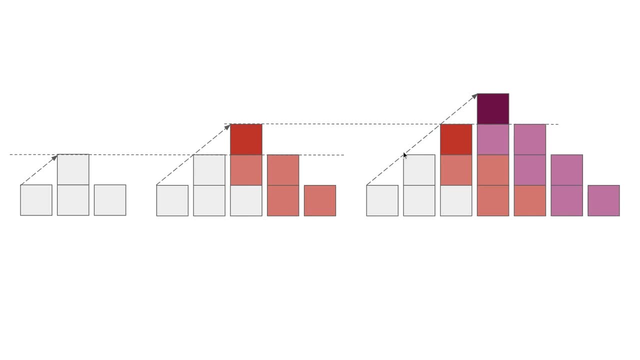 The eighth one. I call it. never give up. It's like you go one more step up every time and you also need to keep the whole shape symmetric so that you can come down to take a break. So you put these extras, extra squares, um under the new top one. Never give up, I call it. 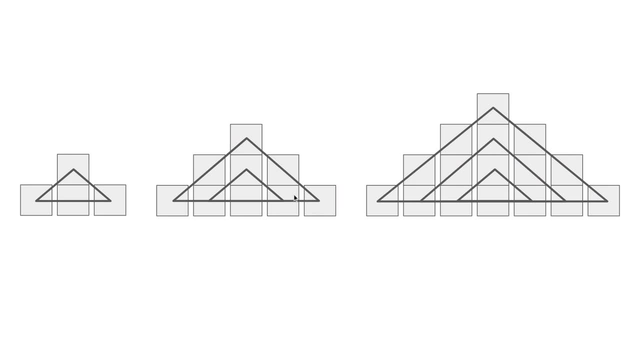 So the ninth perspective, I um we call it similar triangles. The layers can be seen as triangles. This is a different, um similar, um different but a similar perspective. It's another one- It's also called stairway- of that similar triangles. Eleven one: This one is um similar with the never give up one. I call it um stay away. 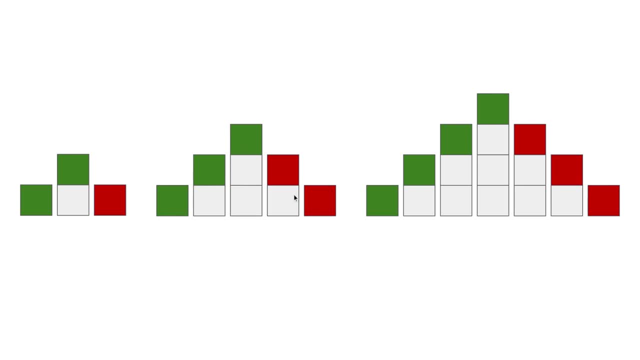 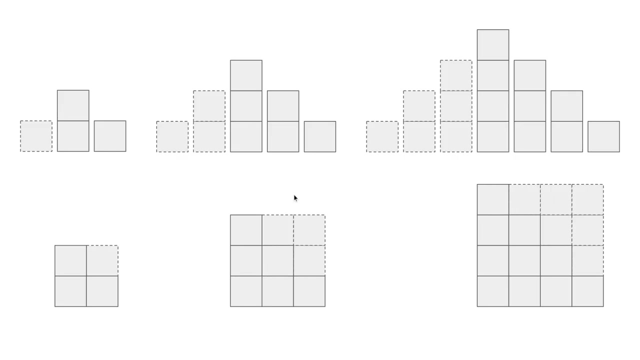 but um access denied. When you reach the new top, you have to come down, so that's called an axis denied. 12th one probably is the most fantastic perspective. just, we could, just we just call it the square. okay, a square can be rearranged to form a large square each time. so at the bottom row. 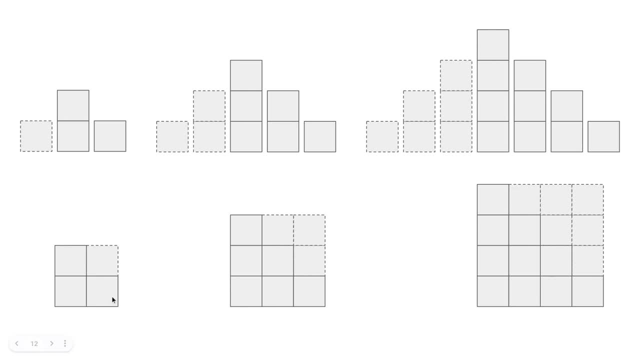 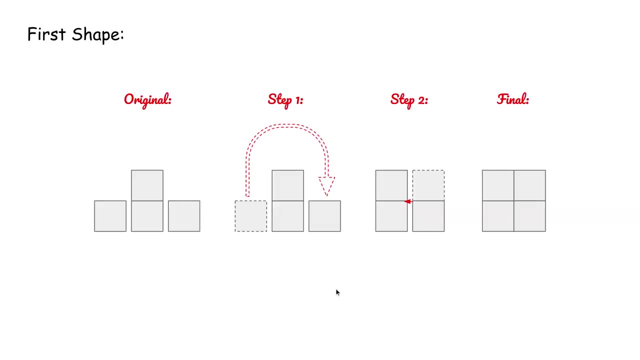 you can see, they can be arranged into these large squares. so how did we do that? we, for example, for the first shape, we do this step one: we move, we are rearranged the dashed squares to its new position so that we can make a new large square. there is a gap between these two. 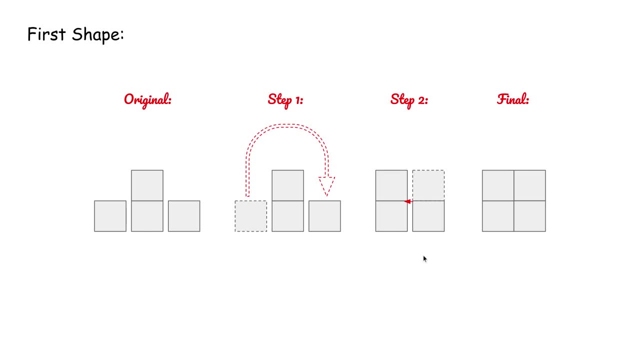 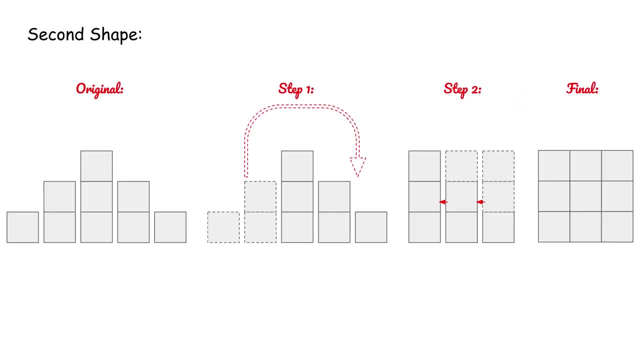 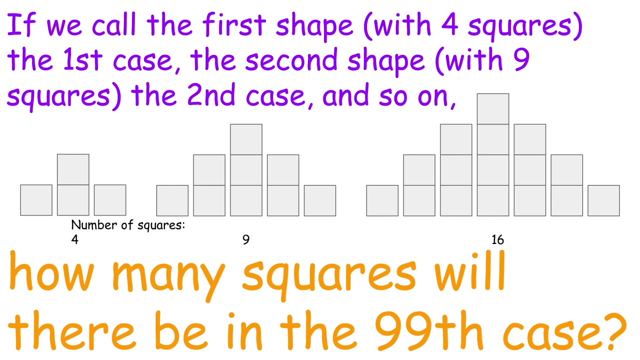 stacks and we kind of compacted them. so make a perfect square, large square. we did do the same process on to the second shape and we also do the same process to the third shape. so here is a question: if we call the first shape with four squares the first case, the second shape with nine, 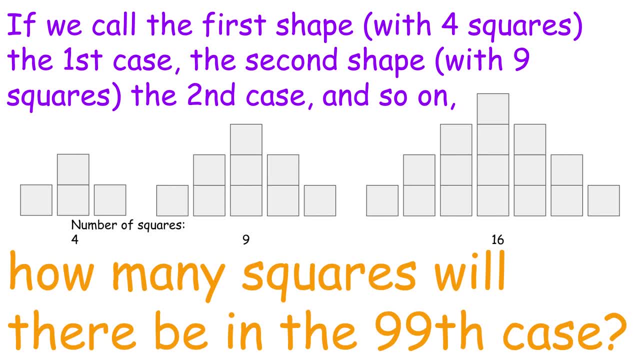 squares, as showing here, the second case and so on. how many squares are there in the first case? many squares will there be in the 99th case? so that sounds like a mathematical question, because we, we shouldn't do, we shouldn't just draw the squares one case by case. that that would be like. 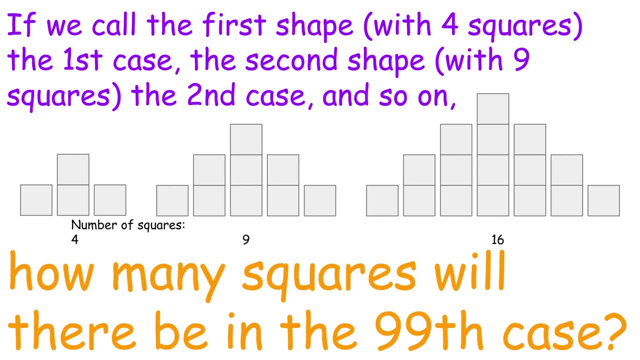 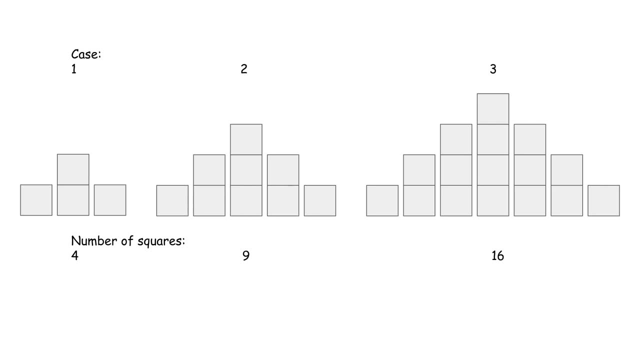 a very tiring and unrealistic right, so it must be some mathematical way to solve it. so we mentioned about the case number, so we list the case number here on the top, so that this we have three cases. so this is case one, this is case two, this k3, and we also count the number of squares at the bottom. for the first case we have three. 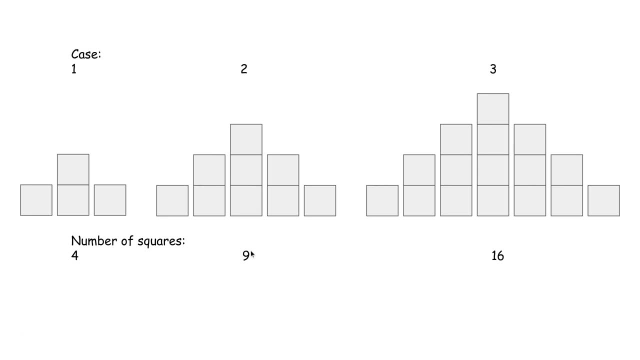 squares. we have four squares, for the second case we have nine squares and for third case we have sixteen squares. so we, as we mentioned about the square perspective, we arrange, we rearrange the squares into a larger square, so we move the dashed square to to form a large square, like we did. 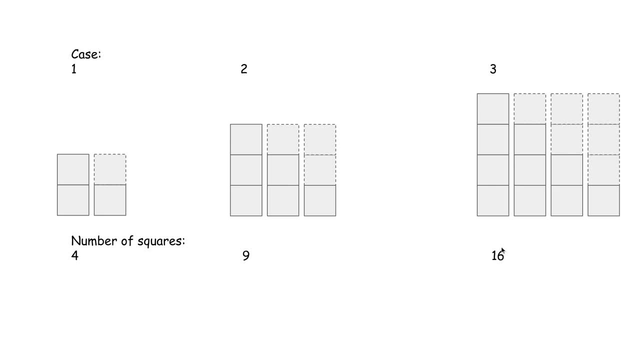 at the last example of a perspective. So we also keep the case number listed here and number of squares listed here and we're going to compact them so that we can get perfect squares, perfect larger squares. So now we have two sets of data. 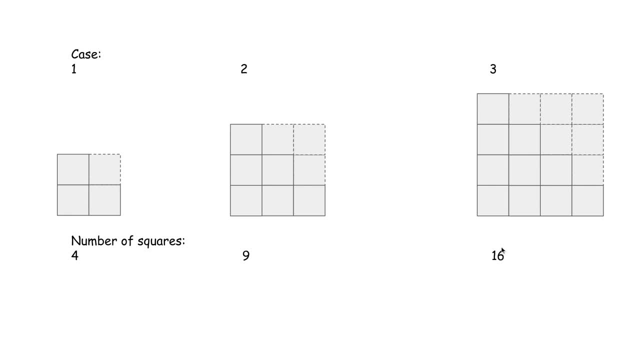 We have number, we have case numbers and we also have numbers of squares for each case. So next I'm going to label. We have- we found that- the number of squares like 4916.. Just sounds like so, for these squares sounds like an area of. 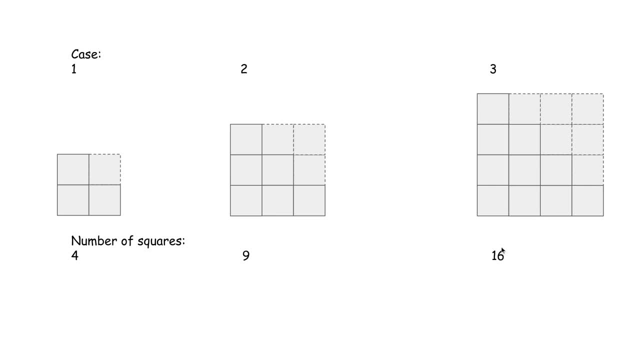 these squares Large squares, So I'm going to label the size length for each large square. So we got a number of squares actually equal to the area of the of these squares- large squares. So we got 4 equals 2.. 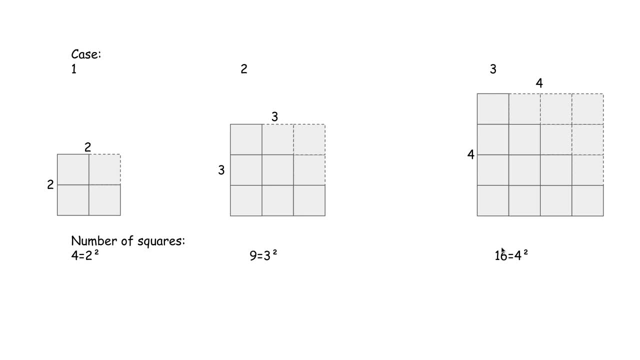 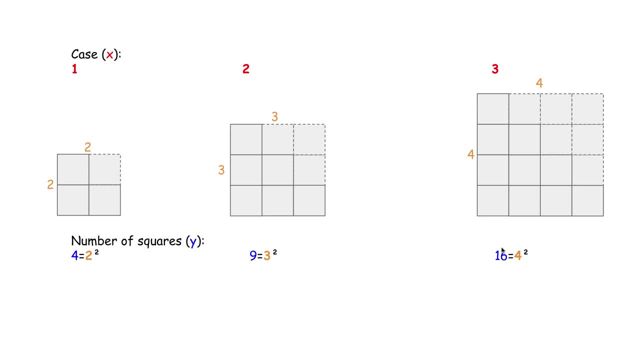 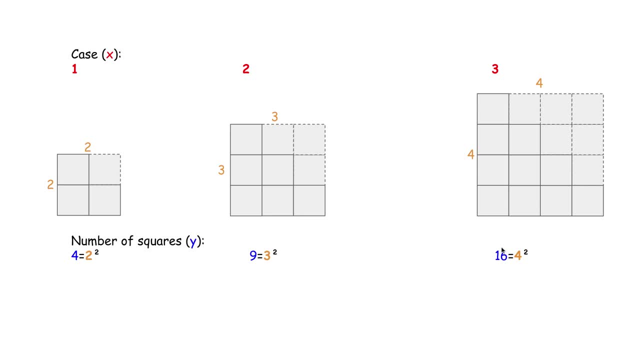 or the difference between the case number and the side length is just one. Okay, so here I'm gonna use X to represent and the Y represent the case number, and I'm going to use Y, and I'm gonna use Y to represent the number of squares. so 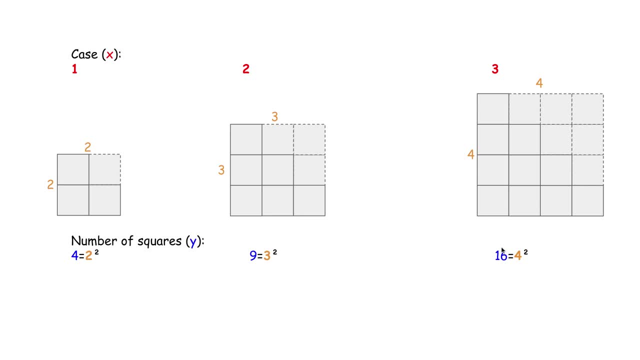 I'm going to make the connection between the case number and the side, between the case number and the site of the length for each larger square and And, like we said, it's just one difference, or the difference is just one, or offset is just one. 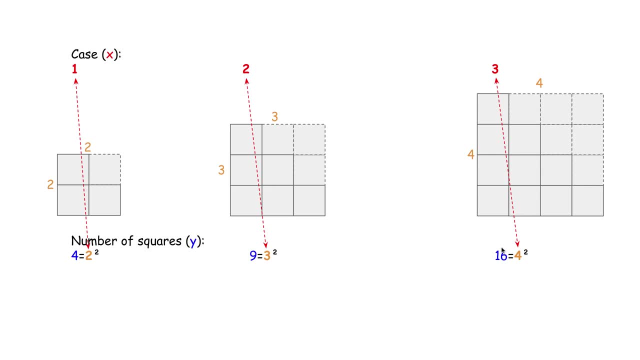 So we're going to use one plus some number to, or we're going to use case number to represent the side length. And see, we're going to use two squared equals one plus one squared. The first one is a case number and because offset is just one, we just plus one. 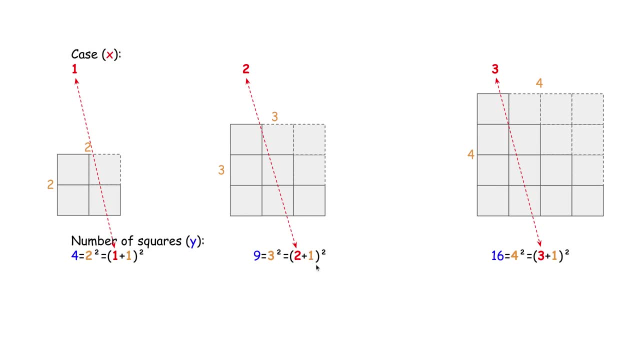 And the offset is always one. it's kind of like constant, And we actually just use the case number plus one. so we got the large square's side length, Okay So. So for the third one, we did the same. So we got three plus one, we got the side length. 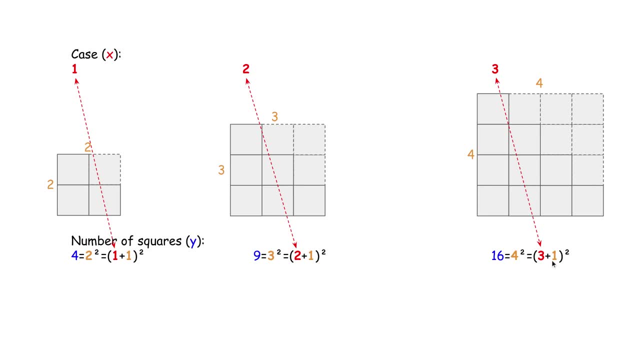 So this is kind of like a pattern here, like a mathematical pattern. here And now we know the constant is one And we kind of got We got some a list of like equations. So we kind of got a number of squares equals case number plus one and parenthesis squared. 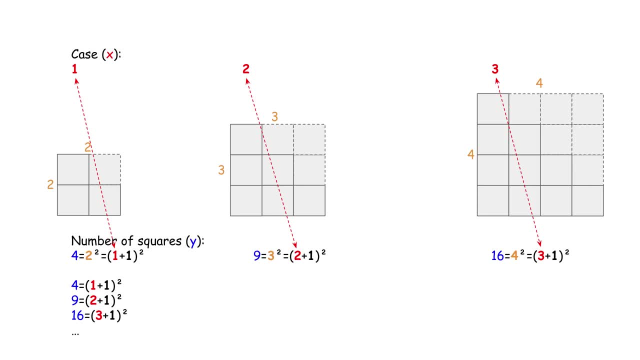 So, for each case, for these three cases, this expression, this is like, applies. And what if? What if we replace this number of squares- four, nine, 16- with just a y And we're going to replace the one, two, three case numbers with x? 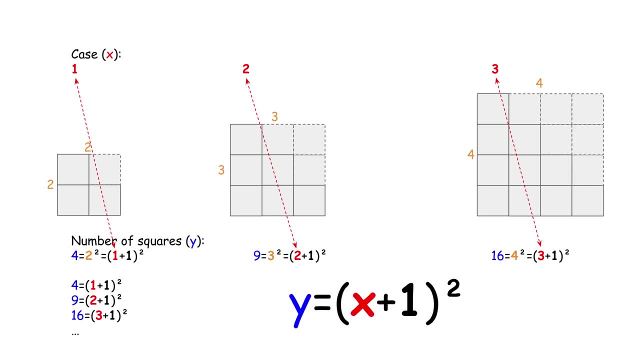 So we got a equation here: Y equals x plus one Pang. This is: This is squared. So now, if x equals 99, that means that's for the 99th case. So we can use this equation to get the number of squares for the 99th case. So it's gonna. 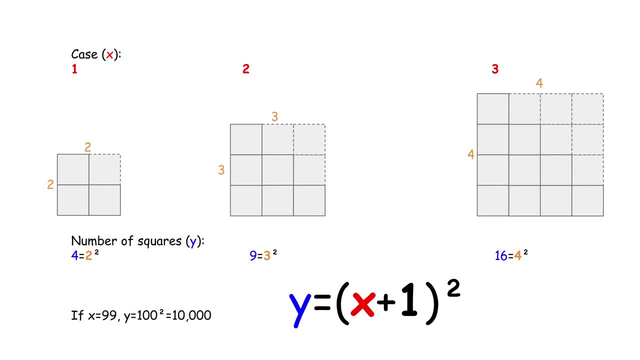 be 99 plus 1 squared, So that 100 squared that's 10,000.. So that's a little bit about the growing pattern. So this is one of the growing pattern, or growing shapes, One example of these growing patterns. So if you are 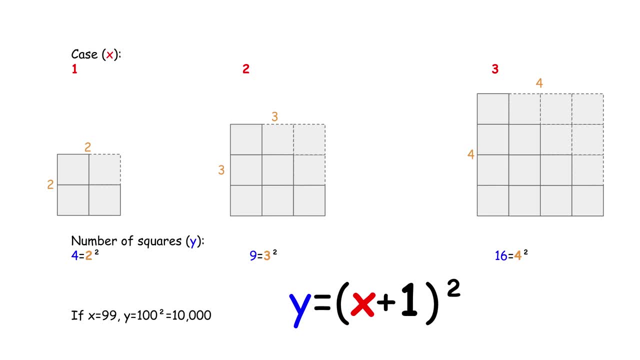 interested, give me a thumbs up or like or subscribe to my youtube channel. Thank you.